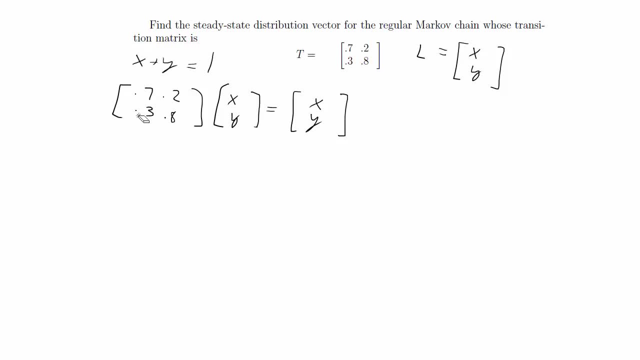 is that x and y has to be equal to 1.. So the probabilities always have to be equal to 1 in the columns, and it's the same thing for the steady-state distribution vector. Okay, so that's going to produce three equations. 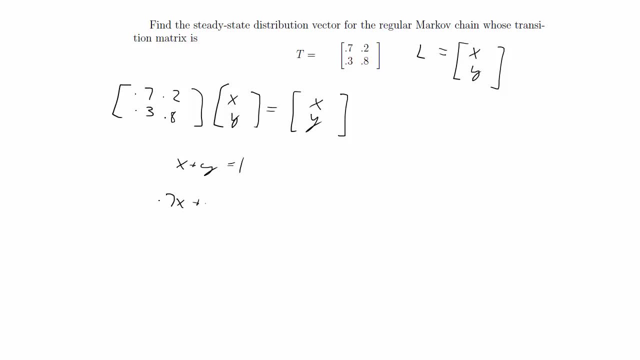 So we have x and y equals 1.. Then we have 0.7x plus 0.2y equals x. just multiplying Then we have 0.3x plus 0.8y equals y. So this gives us three linear equations that we can use to find unique solutions for x and y. 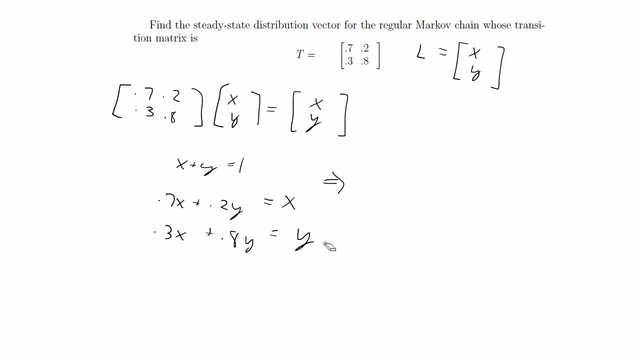 The next thing we want to do is move x to the left side and move y to the left side, so that we can have 0 here and 0 here. Then we can rewrite the coefficients in a matrix, do row reduction, and that will give us the solution. 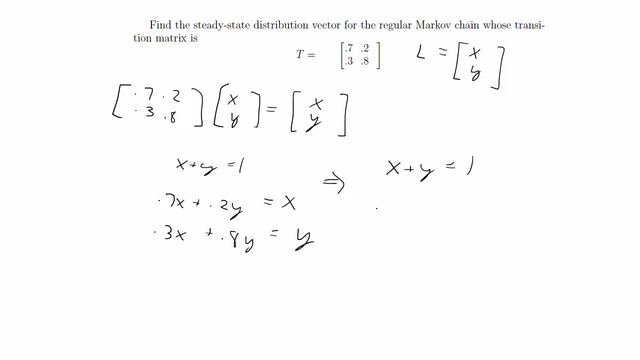 So by that I just mean we have this again. Then we'll have negative 0.3x plus 0.2y, And we have 0.3x minus 0.2y equals 0. Let's rewrite that as a matrix. 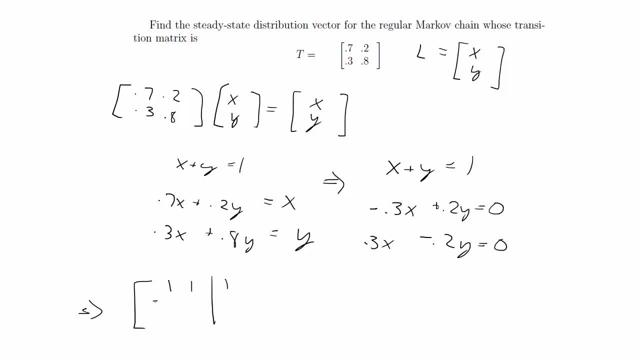 So we have 1, 1 equals 1.. Then we have negative 0.3, 0.2 equals 0. And we have 0.3, negative 0.2 equals 0. If you have to solve this by hand, you would use the Gauss-Jordan elimination method. 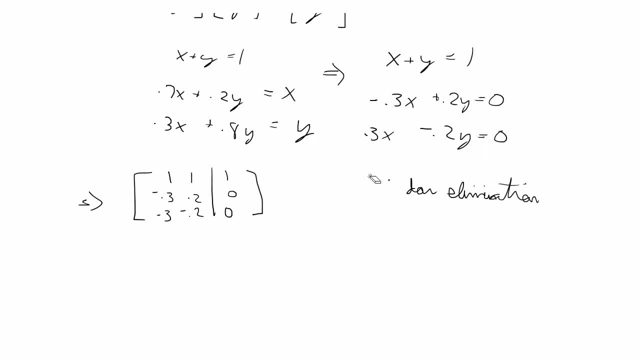 or basically just do row reduction in your calculator. I think I'll do a video on that. I'll talk about how to simplify this in another video, But for now just plug it into your calculator. To put this in your calculator, you just do second matrix, which is the inverse symbol. 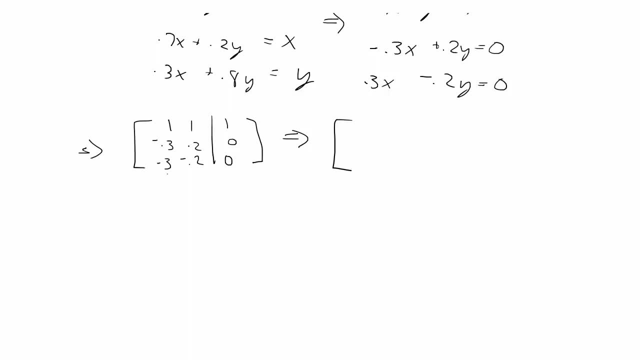 You edit the matrix that you want, Then you go to math. So you want R ref Put in the matrix and then that'll give you the output. The outcome that I get is 1, 0.4, 0, 1.6, and 0, 0, 0.. 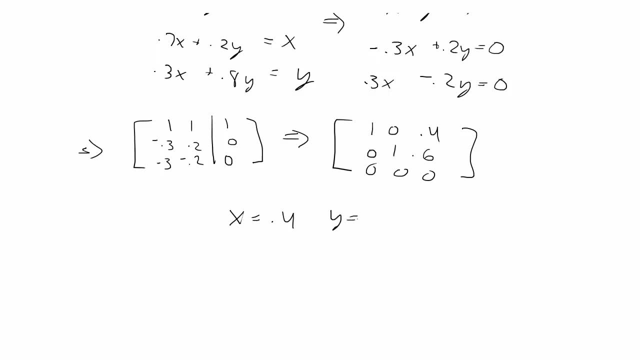 So you can interpret that as meaning x equals 0.4, y equals 0.6.. So your answer, written as the limiting vector or steady state vector, is 0.4, 0.6.. Sometimes, instead of vectors, they're called steady state matrices. 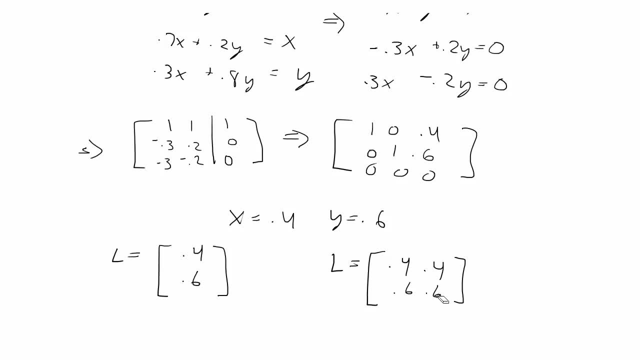 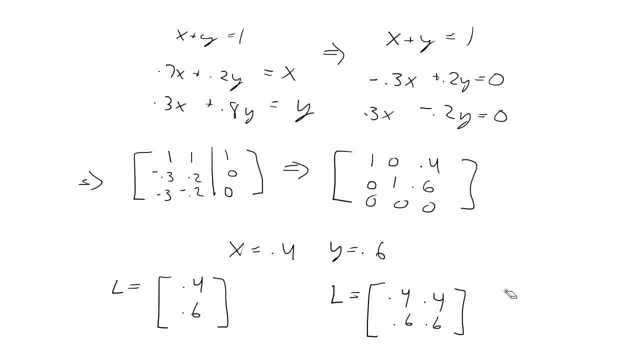 in which case you just write it 0.4,, 0.6, and you just repeat the column again as many columns as is in your transition matrix, But it's the same thing, Okay. so then I'll do the 3x3 matrix example next. 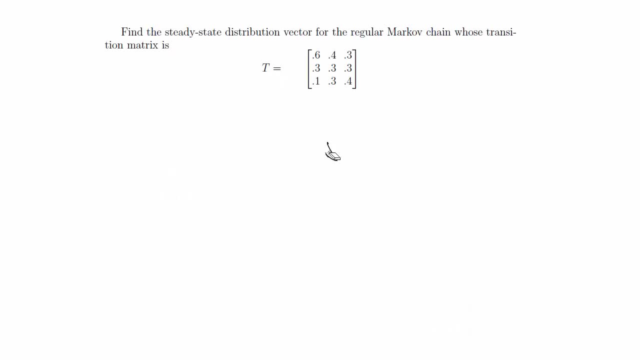 Okay, here's the second example. This one's a 3x3 matrix, but the idea is still the same. So again we're going to want to do TL equals L and then find L. The difference is, this time L will have three variables: x, y, z. 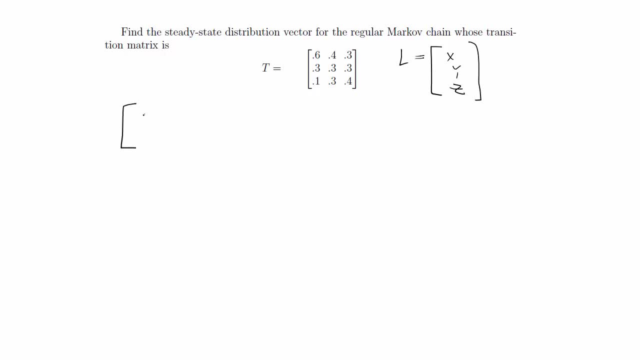 but the concepts are still the same as the other problem. So we have 0.6, 0.4, 0.3, 0.3, 0.3, 0.3, 0.1, 0.3, 0.4 times x y z equals x y z. 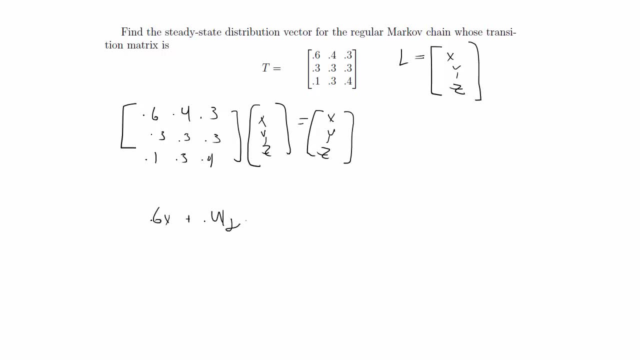 That's going to be: 0.6x plus 0.4y plus 0.3z equals x. 0.3x plus 0.3y plus 0.3z equals y. 0.1x plus 0.3y plus 0.4z equals z. 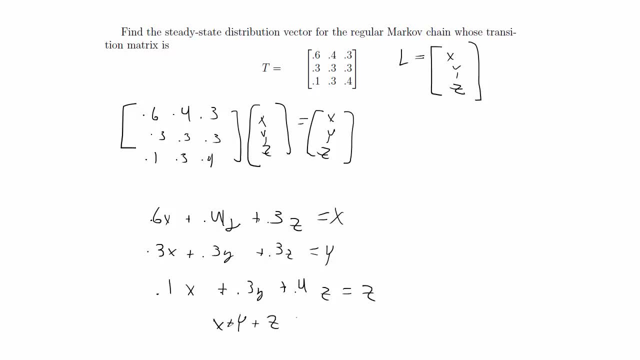 and we also have: x plus y plus z equals 1.. Rewriting that we get negative: 0.4x plus 0.4y plus 0.3z equals 1.. 0.4x plus 0.4y plus 0.4z equals 1.. 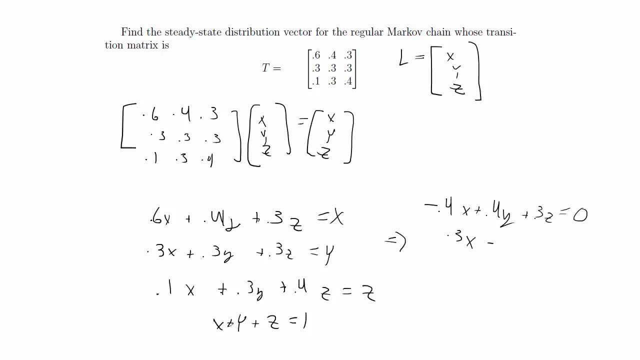 0.4x plus 0.3z equals 0.. We get 0.3x minus 0.7y plus 0.3z equals 0.. We get 0.1x plus 0.3y minus 0.6z equals 0.. 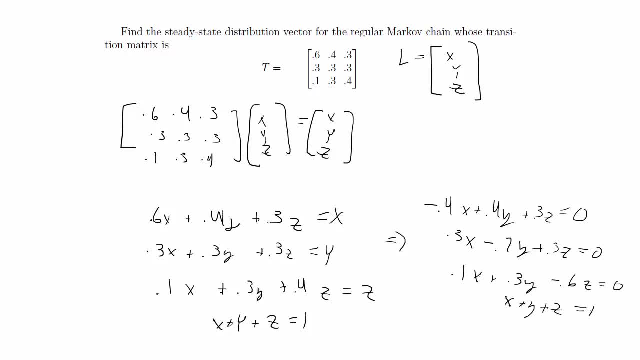 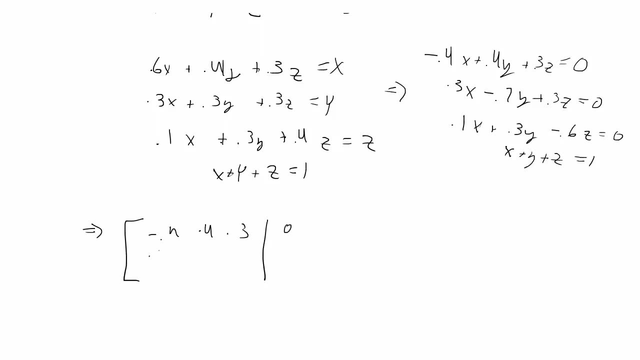 And we have x plus y plus z equals 1.. Rewriting that as a matrix, we get: negative 0.4, 0.4, 0.3 equals 0.. 0.3, negative 0.7, 0.3 equals 0.. 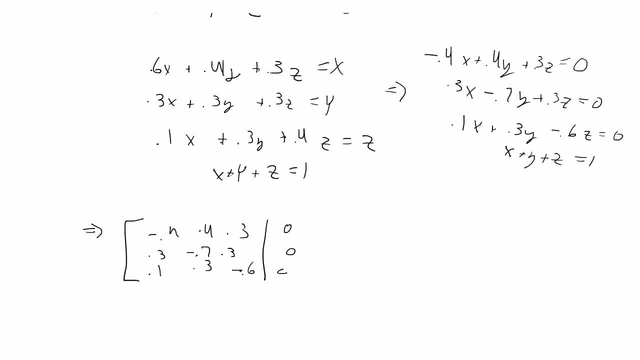 0.1, 0.2, 0.3 equals 0.. 0.1, 0.2, 0.3 equals 0.. 0.2, 0.3 equals 0.. 0.3, negative 0.6 equals 0.. 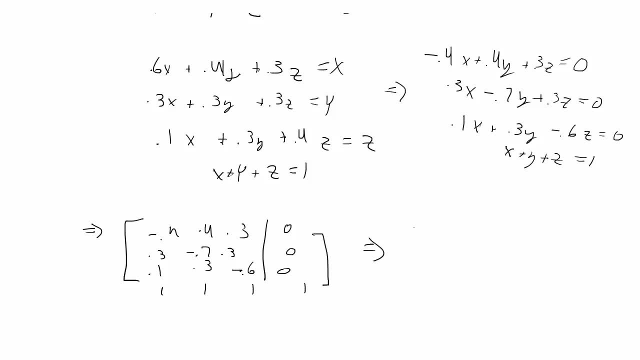 And 1,. 1, 1 equals 1.. Let's put that in the calculator and do row reduction. The values in the matrix table that it will give you are in decimals. If you hit math and then 1,, that will change the answer to a fraction.